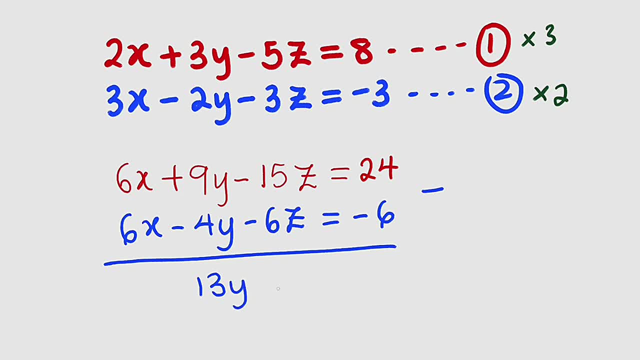 tartan y right. So we have tartan y right here. Then we have negative 15 minus minus 6, which is the same thing as negative 15 plus 6, which is negative 9z, And this is equal to this minus minus this, which is the same thing as 24 plus 6, which is equal to 30. So we have 30 here. 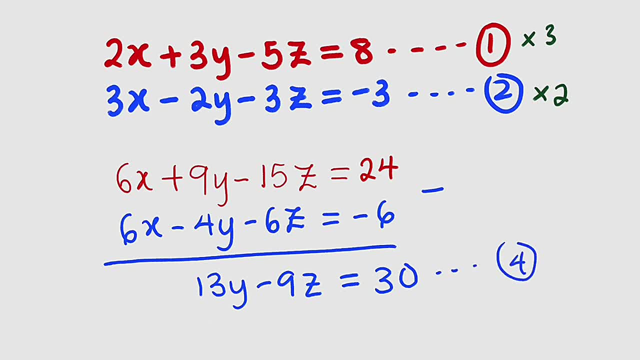 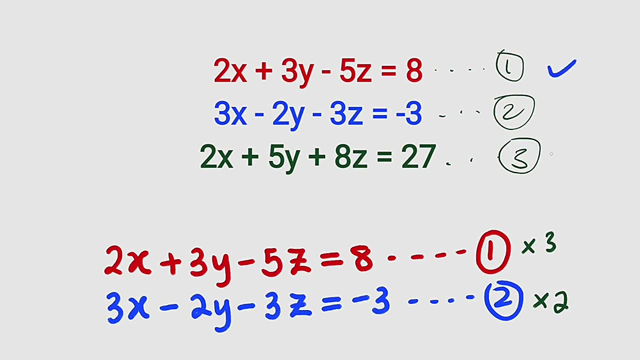 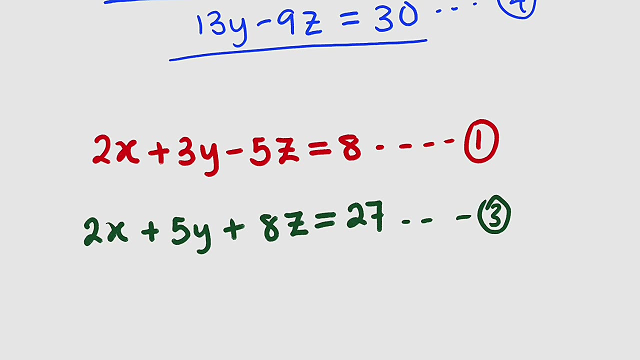 We can call this as equation number four. Now I would like to compare equation one and equation number three, which is this and this: also to eliminate x. All right, here is our equation one and equation three. We would like to eliminate x as well. so we're going to subtract, If we subtract. 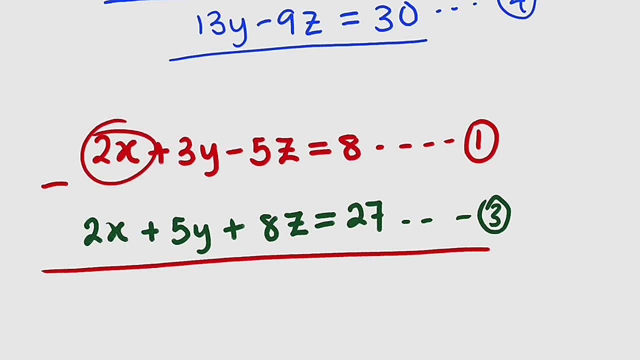 this into the math column, we will find that we have 2x minus 2x, which is going to give us zero. Then we move to y. we have 3y minus 5y, which is going to give us negative 2y. 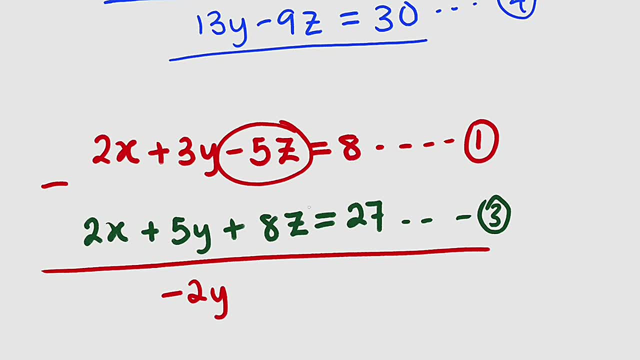 Then we have negative 5z minus 8z, which is going to give us negative 13z, Negative 13z. And lastly, we have 8 minus 27, which is going to give us negative 19.. So this is our equation number 5.. 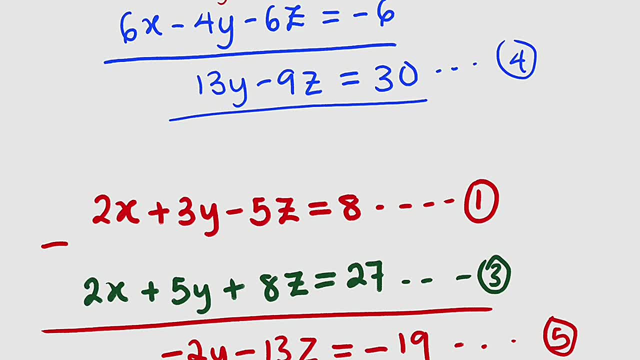 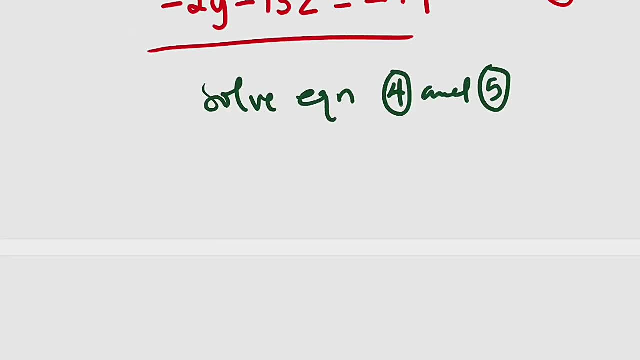 Now I would like to relate equation number 4 and equation number 5 and solve them simultaneously as well. So we want to solve equation 4 and equation 5 together. Equation 4 is 13y minus 9z, equal to 30.. 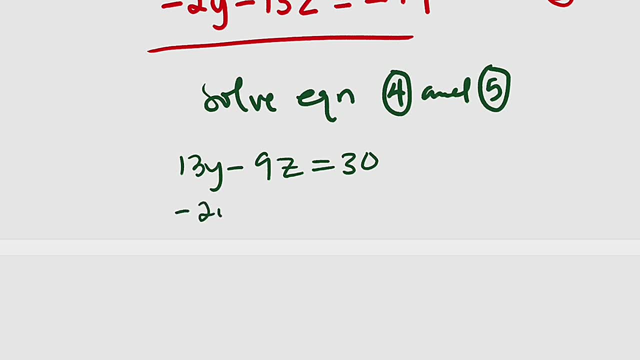 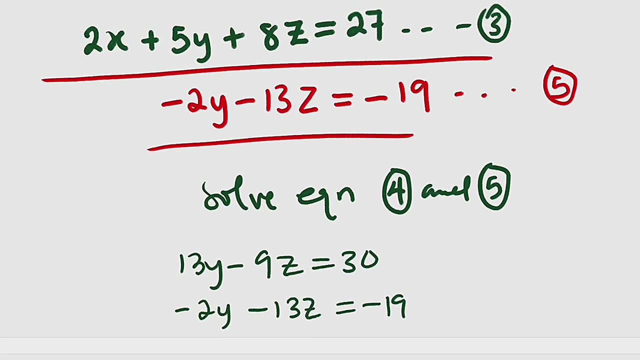 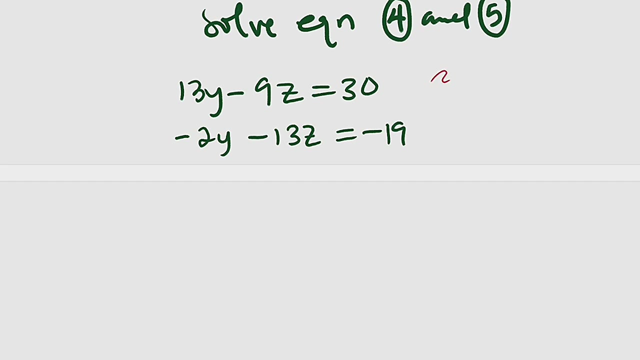 And the other equation, which is equation 5, is negative 2y, negative 13z, equal to negative 19.. Let me confirm: Yes, Since we are dealing with elimination, I would like to eliminate y here by multiplying this equation by 2 and multiply this equation by 30. 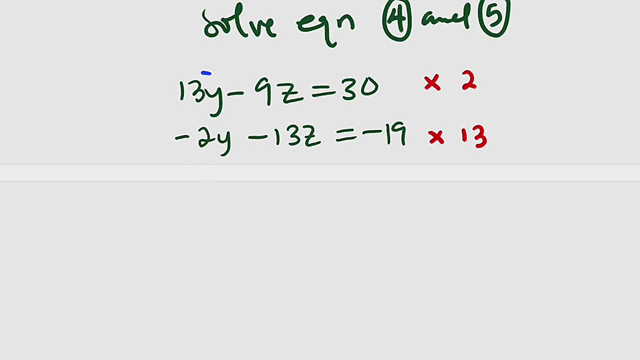 All right, Let me rewrite the equation: 2 multiplied by 30 will give us 26.. So we have 26y here. minus 9 times 2 is 18z. This is equal to 30 times 2, which is equal to 60.. 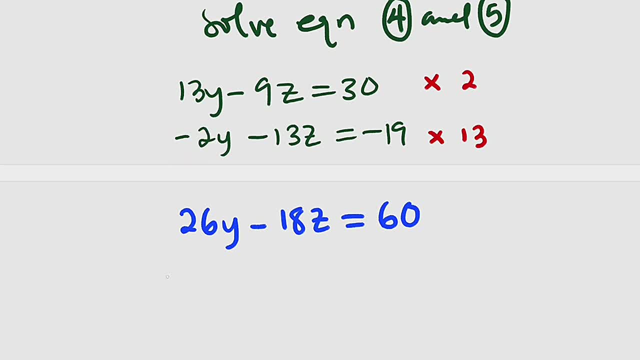 Then if you multiply negative 2 with 30, you're going to obtain negative 26y minus 30 times 30 is 169.. So we have 169.. Z here. this is equal to negative 19 times. starting will give us negative 247.. 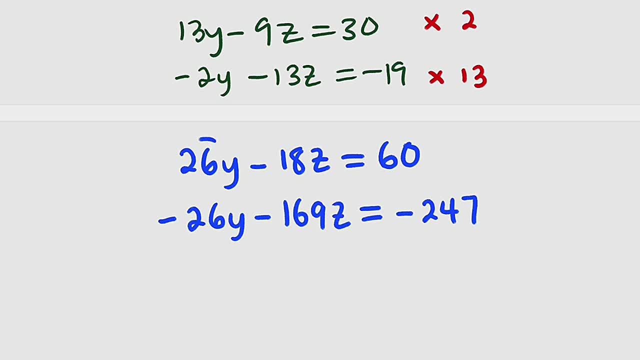 All right, Now we're going to add the two equations because you can see they have opposite coefficients. If we add, we are going to get 0y. So you add this, you get 0y. If you add negative 18 and negative 169 together, you're going to obtain negative 169.. 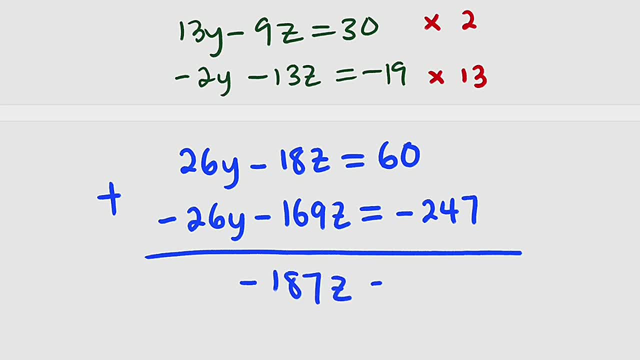 All right, All right. So this is equal to negative 187z, which is equal to 60 plus negative 247,, which is the same thing as 60 minus 247, will give us negative 187.. To find z, we're going to divide both sides by the coefficient of z. 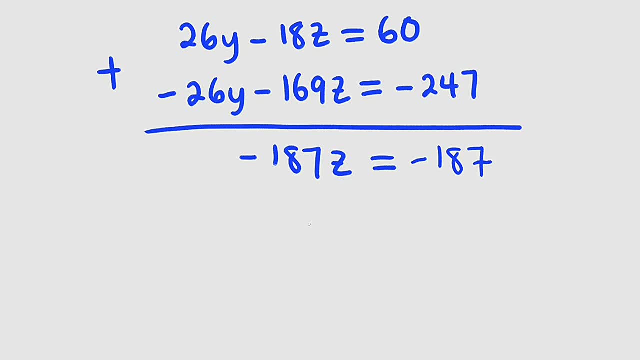 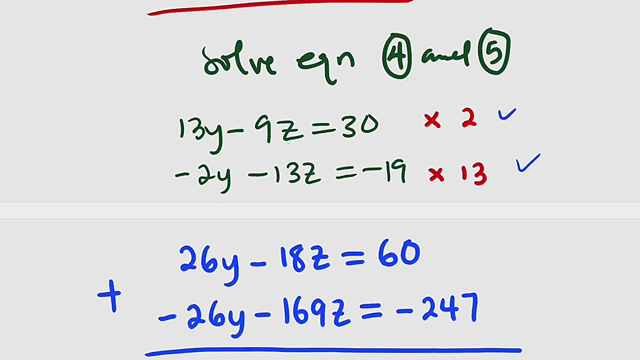 You can see, these two numbers are exactly the same. Therefore, z is equal to 1.. We have obtained the value of z, All right. Now you can plug this z into one of these two equations. All right, Let me use this equation which is starting: y minus 9z equal to 30.. 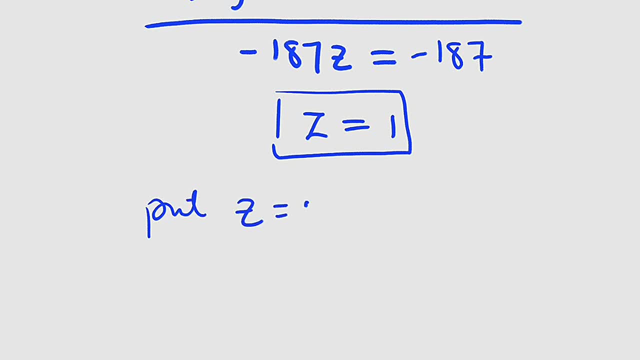 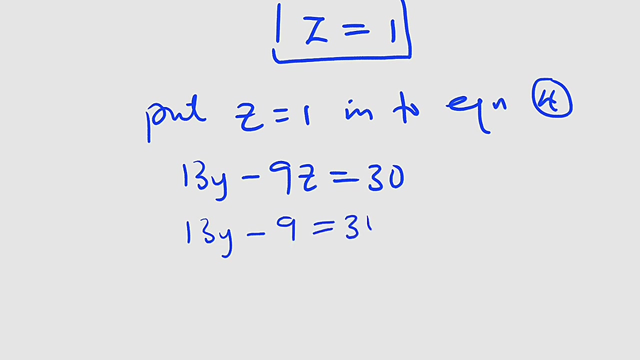 So put z, equal to 1, into equation number 4.. And equation number 4 is starting y minus 9z, equal to 30. Wherever I have z, I'm going to replace it with 1.. So therefore, this is starting y minus 9 times 1, which is 9, equal to 30. 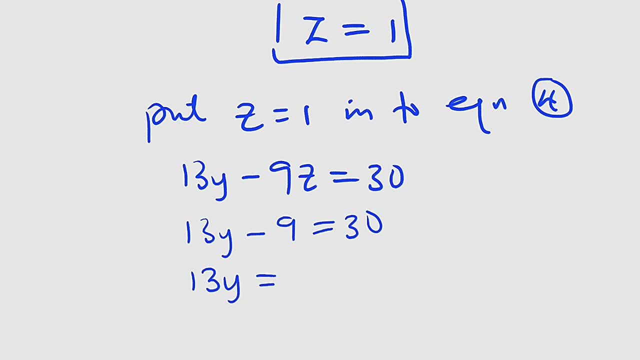 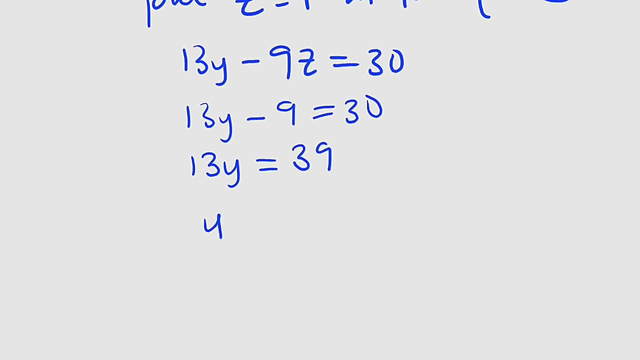 Take 9 to the other side, We have starting y equal to 30 plus 9,, which is 39. You should divide both sides by 30. y will be equal to 3, because starting 9 divided by 30 is equal to 3.. 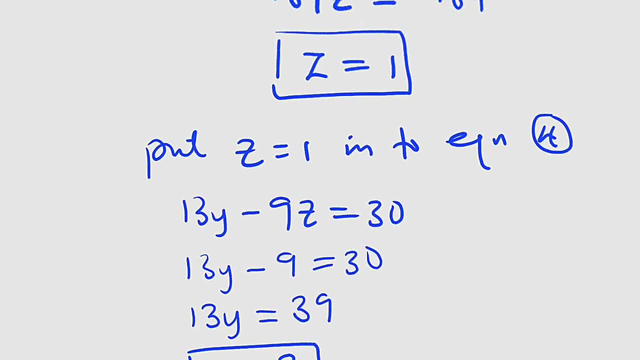 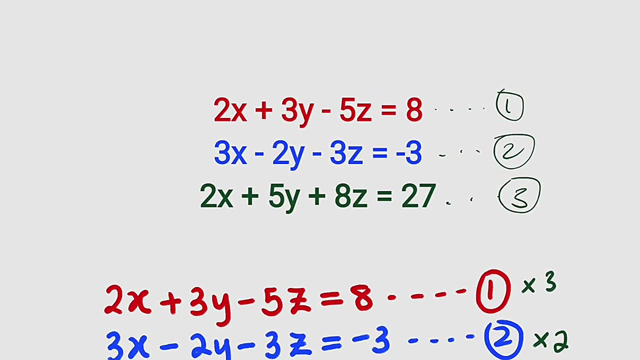 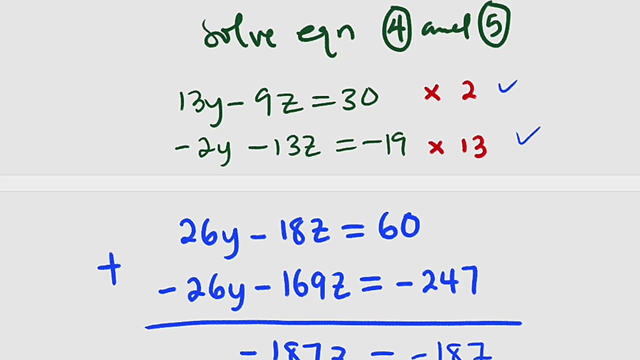 Now we have the value of y and the value of z. We can take these two solutions and substitute them. We can substitute them into either equation 1 or equation 2 or equation 3.. Let me use equation 1, which is 2x plus 3y minus 5z, equal to 8.. 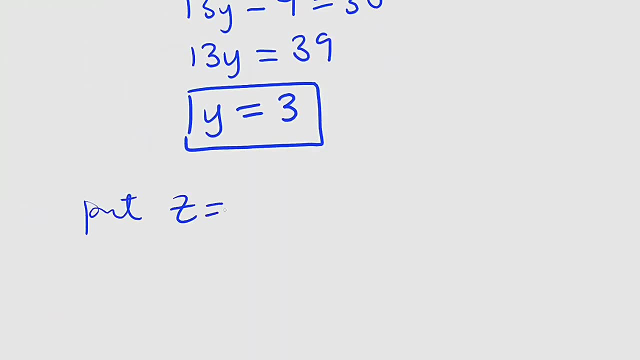 So put z, equal to 1, and y equal to 3 into equation number 1.. And equation number 1 is 2x plus 3y Minus 5z, equal to 8.. We are looking for x, So we have 2x plus 3 multiplied by y. 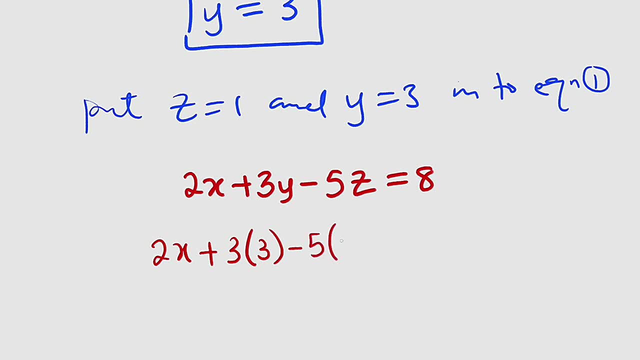 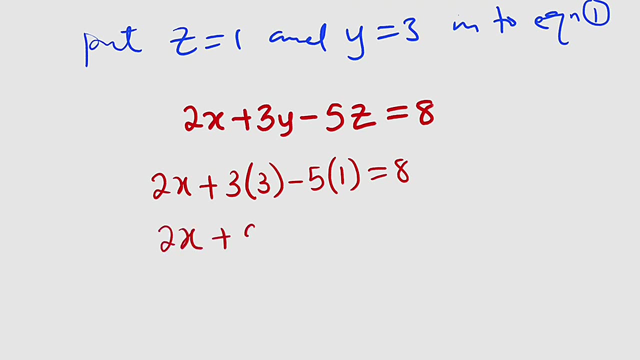 y is 3.. Minus 5 multiplied by z but z is 1. And this is equal to 8.. We have 2x plus 3 times 3, 9 minus 5 equal to 8.. You know that 9 minus 5 is 4.. 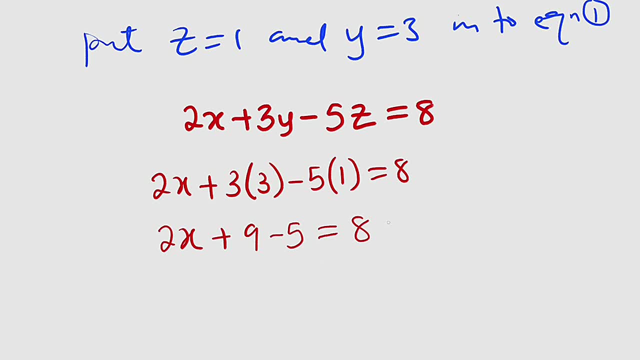 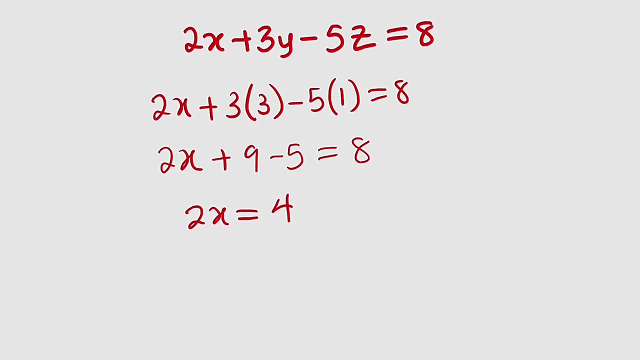 You can take 4.. The other side, it becomes negative. 8 minus 4 is 4.. Therefore, 2x is equal to 8 minus 4, which is 4.. If you divide both sides by 2, you have x to be equal to 2.. 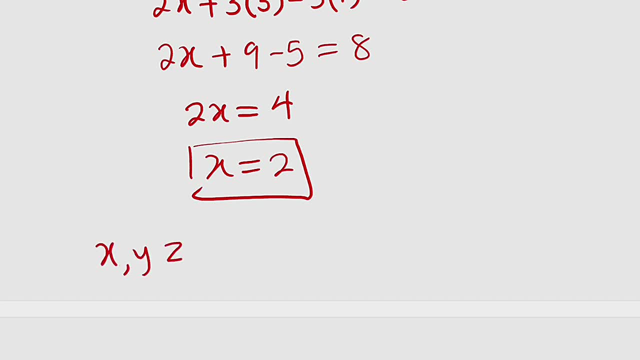 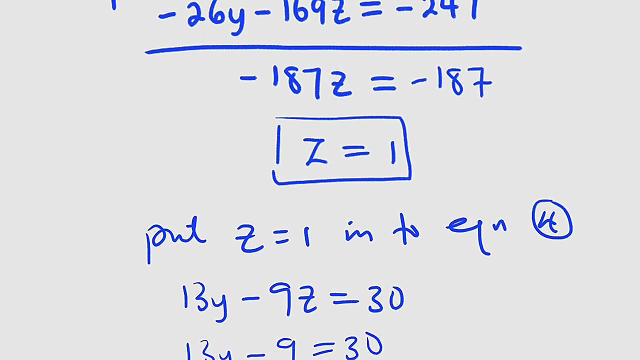 And hence we conclude that x, y, z are nothing but x equal to 2,, y equal to 3, and z equal to 1.. And hence this is the solution to this problem. Thank you for watching. Do share to your learning colleagues. 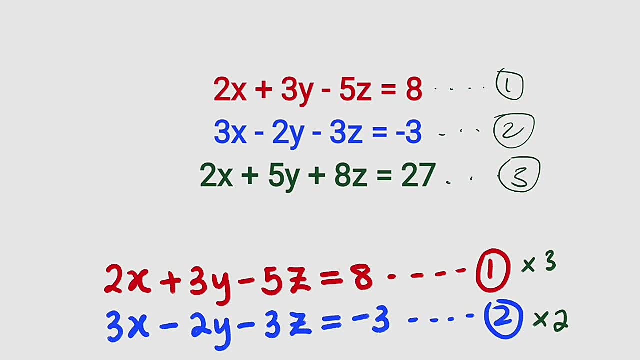 And don't forget to subscribe to my YouTube channel for more exciting videos. Bye-bye, Bye-bye. 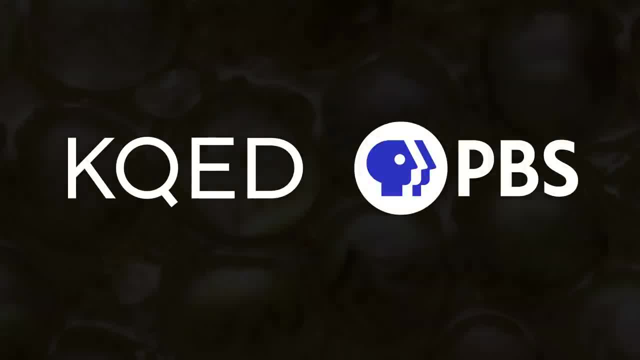 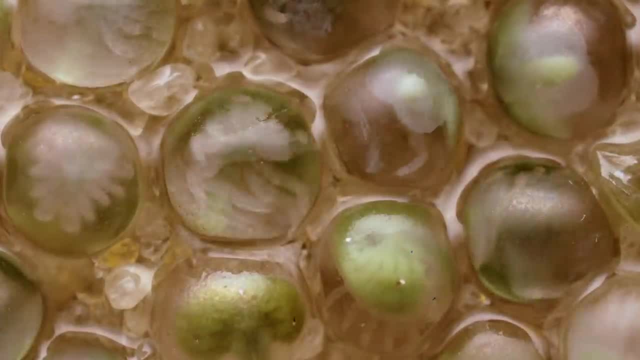 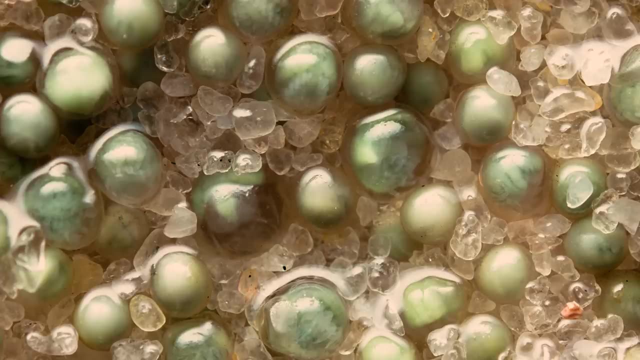 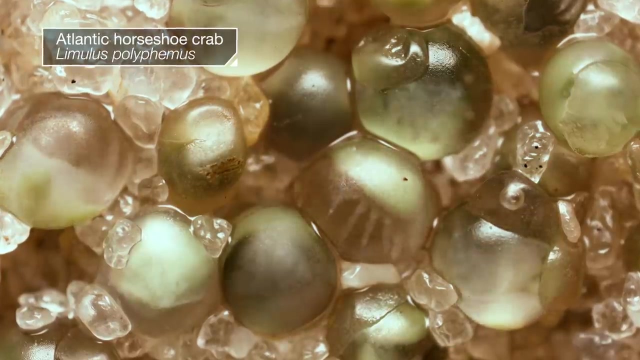 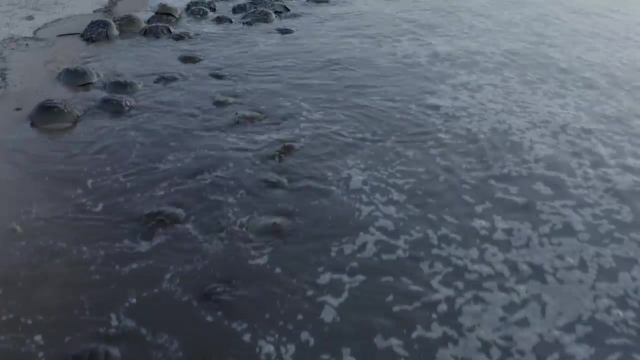 These delicate otherworldly creatures are just starting their lives twitching and twirling inside their translucent homes. They're baby horseshoe crabs preparing for the moment they can break free. It all started two weeks ago when the tides were at their highest. Horseshoe crabs emerge.